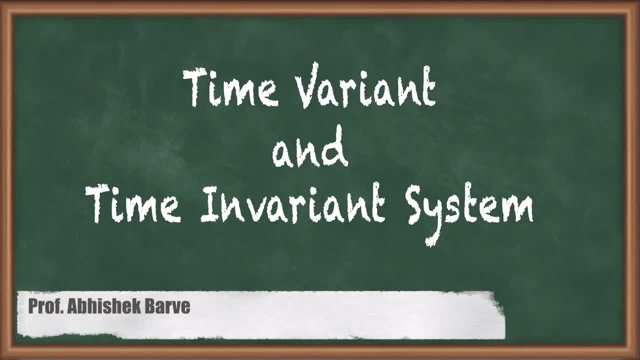 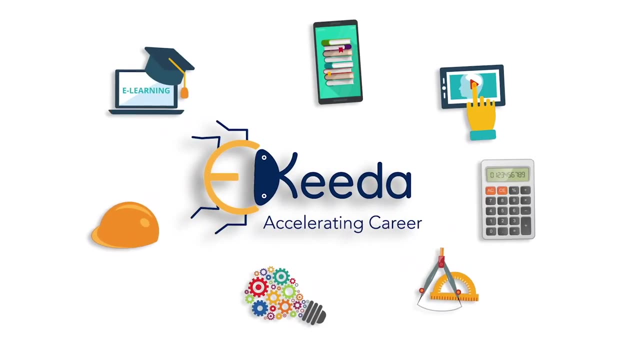 Hello friends, in this video we will be learning Time Variant and Time Invariant system. In fact, we will follow a particular procedure to identify whether the given system is Time Variant or Time Invariant. Let us begin. Let us understand the definition first. 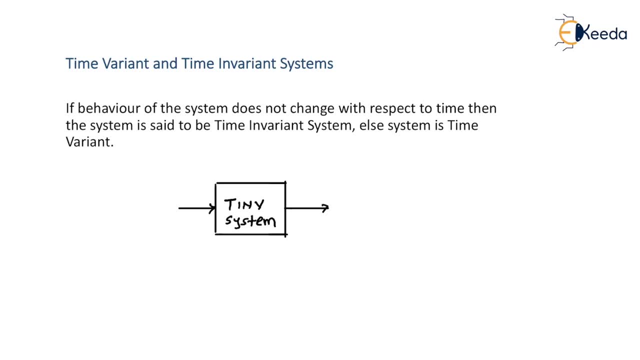 If behavior of the system does not change with respect to time, then the system is said to be Time Invariant system. So, as the name implied, it is something which is not varying with respect to time. That is, properties of a given system if they are not varying or not changing with. 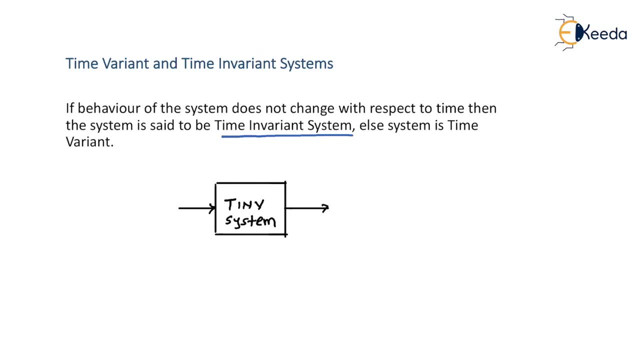 respect to time, the respective system is called as Time Invariant system. But on the opposite side, if there is a particular system whose parameters or whose properties are changing with respect to time, then the respective system is called as a Time Variant system. 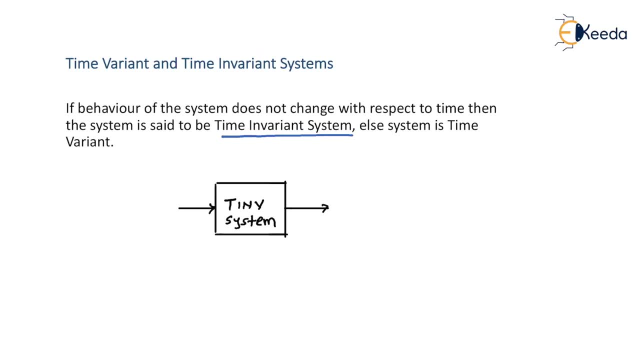 Right. For example, let us say we have a Time Invariant system here to which suppose you have applied this sort of input. So let us say you have applied some gate pulse here within the duration from 0 to 2, this is your x of t. and let us say you are getting y of t. 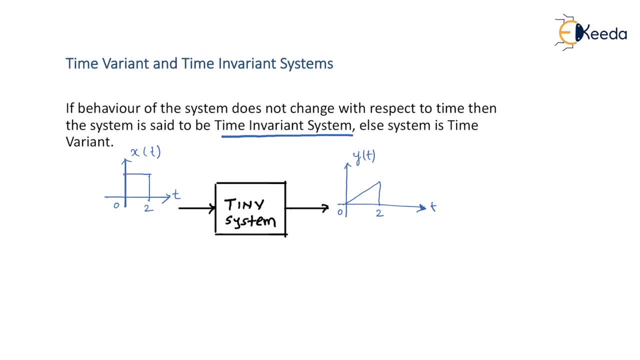 So this is just an example where you are getting y of t here. So let us say, for this particular x of t, let us say, after applying this x of t, after processing on x of t, this system is producing this sort of output. 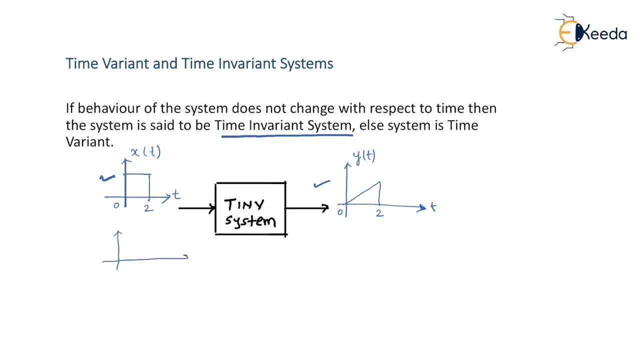 For example, if same x of t is, let us say, delayed by some amount, let us say by 1, then it becomes x of t minus 1.. Right, Therefore, what will happen? The above gate pulse gets delayed by 1 second. 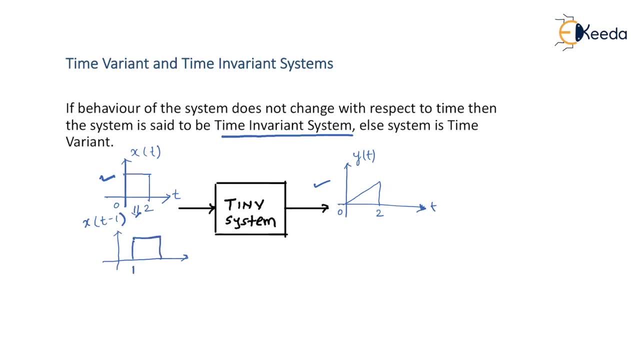 Right, Then a new gate pulse I can draw like this, ranging from t equal to 1 to t equal to 3.. Again having same amplitude, because I have operated only on time scale, Then it is expected, output y of t should also get delayed by same amount. 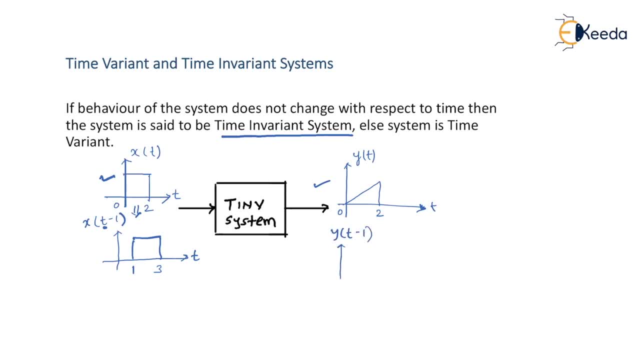 Then you must get y of t minus 1, according to Time Invariance property. Therefore a similar triangle you will get, but then it will start with t equal to 1.. And it will end at t equal to 3.. 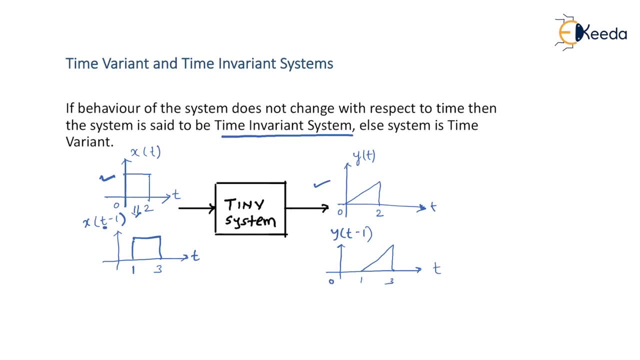 Is that right? See, suppose to give you an example, suppose you are buying an amplifier. Then today, if it is acting as an amplifier, after some days also, it should act as an amplifier and it should amplify the signal with same amount of gain. 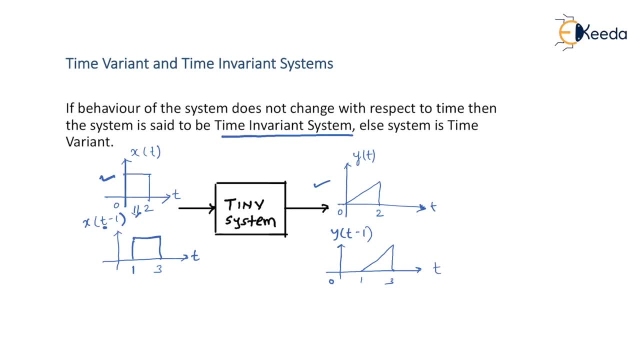 And only then I will say that for that respective amplifier gain of the system is not changing with respect to time. Whatever gain that you are having today, You will get same gain tomorrow, may be day after tomorrow or may be after few months also. 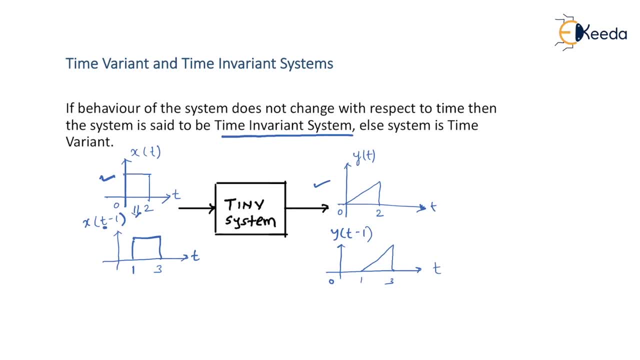 Right, Because the property of that system is not varying with respect to time. Only the reason why I can say that a particular system is a Time Invariant system. Otherwise, if it is varying with respect to time, then the respective system would be called as a Time Variant system. 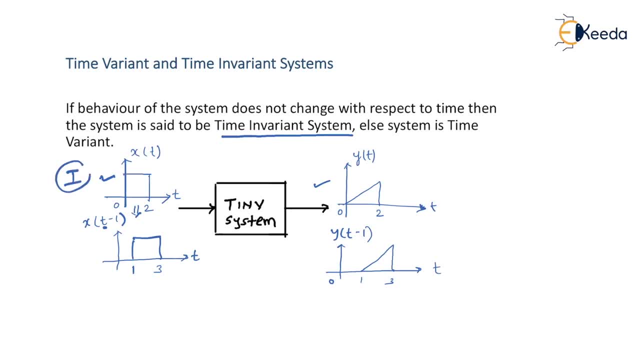 For example, now in case number 1, I have applied this x of t, for which I am getting respective y of t, Right, Same x of t, Right, Same y of t. At the same time, Let's say you are applying tomorrow. 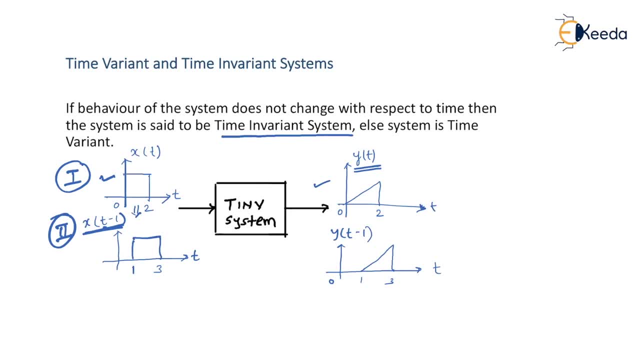 That's the reason why, in second case, what I have done, I have delayed the same x of t by amount 1.. Right, Then you will be getting same y of t not today but tomorrow, because you are applying this pulse tomorrow. So this triangle you are supposed to get tomorrow. 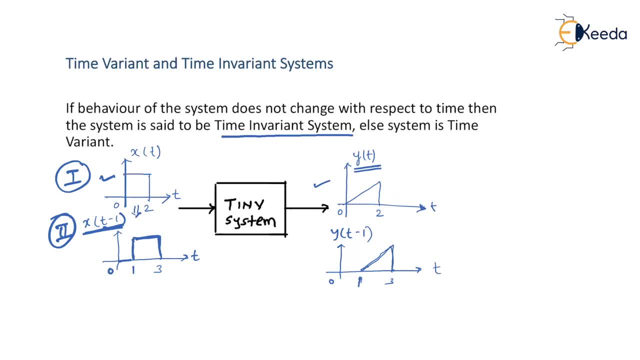 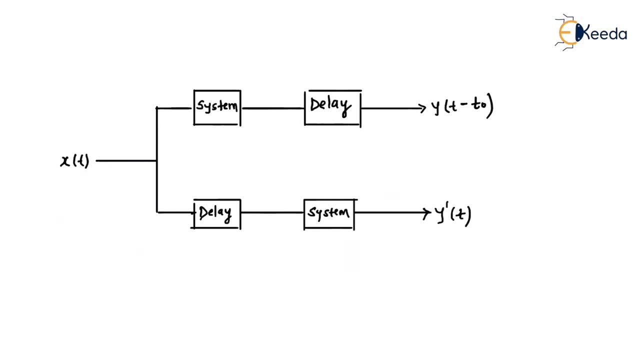 It means it is getting delayed by the same seconds or same time. That's the whole idea of Time Invariant system. So this block diagram will make you a concept. So this block diagram will make you a concept. So this block diagram will make you a concept. 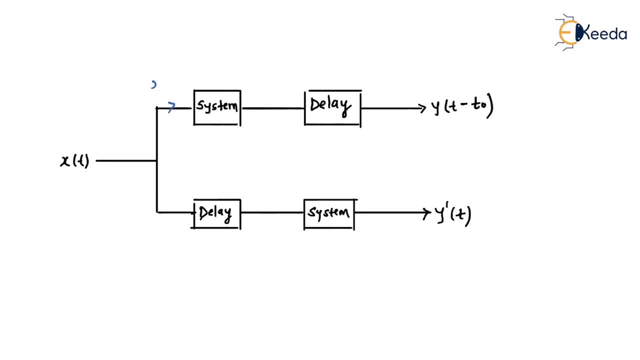 Let's say this: x of t is applied to a particular system After processing on x of t, of course it is going to produce some output. Let's say y of t. As you can see there is a delay block, Assuming it is delaying the input signal by t0 amount and therefore if input is y of t, 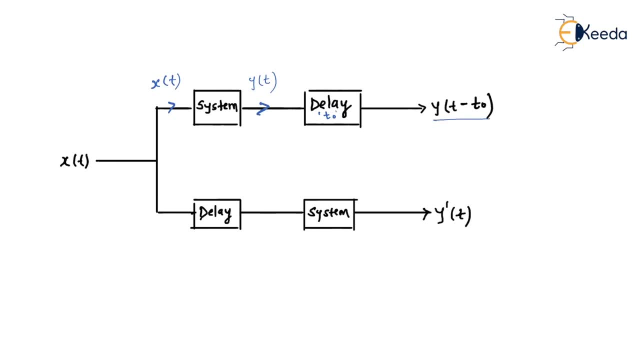 output would be y of t minus t0.. Right, As you can see here, the same x of t is applied here. As you can see here, the same x of t is applied here. If you observe carefully, this delay block and system block are exchanging their positions. 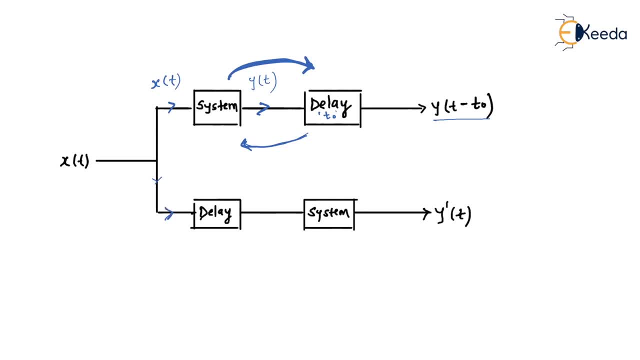 So instead of applying input to system first, it is applied to delay block first and thereafter output of delay is given to the system. Therefore, let's say it is quite a similar delay block which delays the given input by t0 amount. So if input is x of t, I can see that after delaying it becomes x of t minus t0. 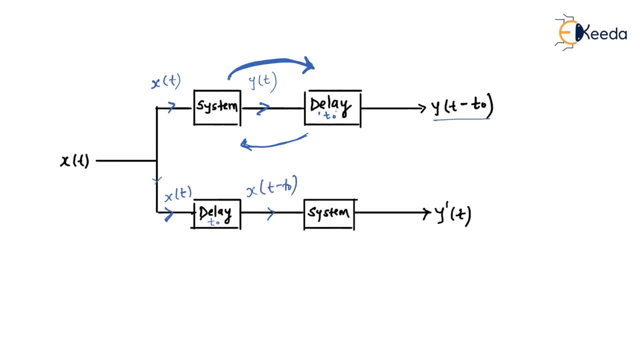 becomes x of t minus t naught. and let's say now it is applied to the system assuming some output, that is, y dash of t. if this y dash of t is equal to y of t minus t naught, that means if these two inputs, after comparison, we find that they are equal, then the respective system is called as. 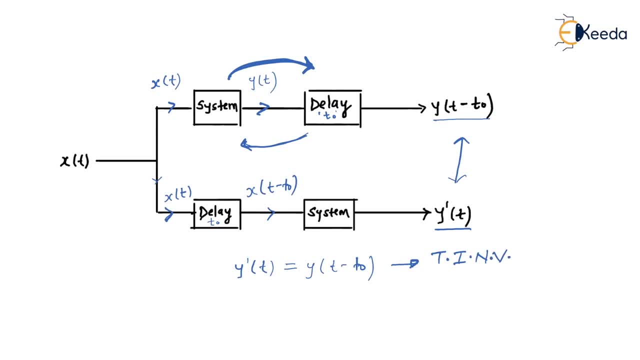 a time invariant system. if y dash of t is not equal to y of t minus t naught, then the respective system is called as a time variant system. so whether it is time invariant or time variant system, it depends whether y dash of t is equal to y of t minus t naught or not, right? so what i've? 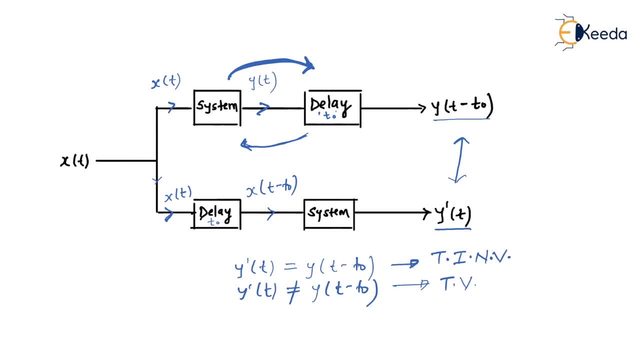 done. see once again: in first case x of t is applied to the system and thereafter it is delayed by t amount. output becomes y of t minus t naught. in second case, x of t is first of all delayed by t naught amount, so it becomes x of t minus t naught. so now input of system is not x of t but x of t minus t naught. 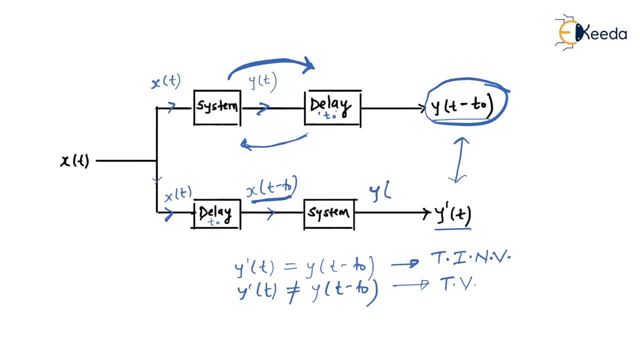 then we believe that output should be also y of t minus t? naught, because that's the whole idea of time invariant system. so for any time invariant system, let's say, if input is x of t, output is y of t, and if input is x of t minus t naught, then output should be y of t minus t- naught, only right. 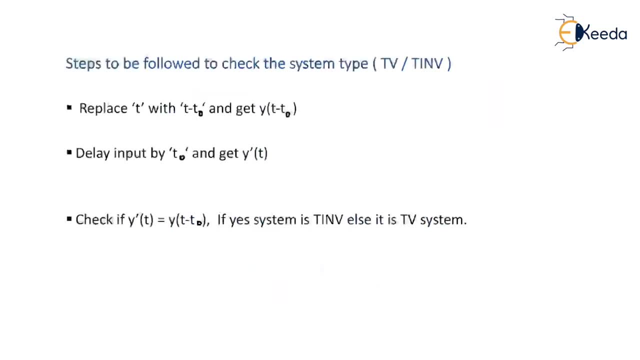 okay, that's everything for today. so let's go through the steps to check the system, whether it is time variant or time invariant. in first step, you have to replace t with t minus t naught and you have to get y of t minus t naught. it is because most of the time y of t is expressed as a function. 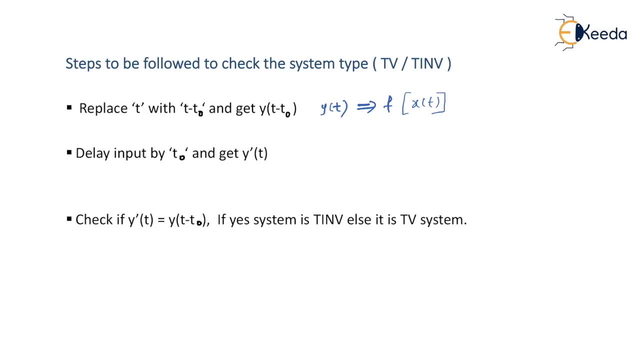 of x of t. so whenever you replace t with t naught, naturally this becomes y of t minus t naught. so So whatever answer comes, it would be y of t minus t naught, and then we will name this equation as equation number y. In second step you have to delay your input by t naught amount. So for example: 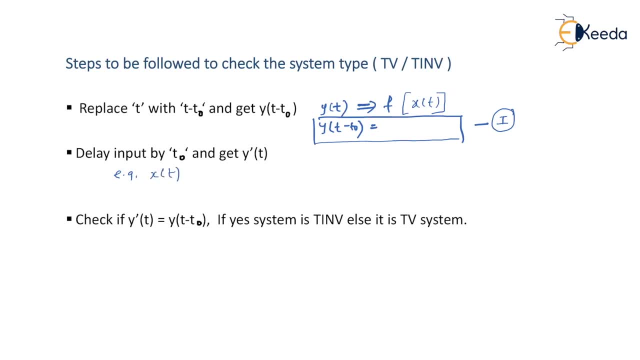 if previously input was x of t, then you have to make it x of t minus t naught, So you have to only delay the input, and then you have to calculate output, and that output is what we called as y dash of t, for which you will be getting a particular equation. Let us assume, 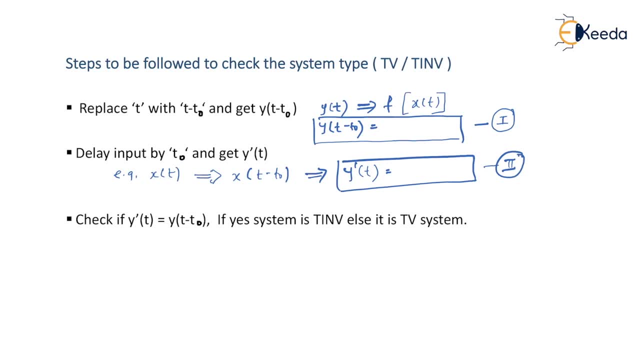 this is equation number two and, of course, what we have done in the block diagram in the previous slide same we are doing it over here, right? Then we are going to check whether y dash of t and y of t minus t naught are equal to each other. If yes, then the system is time invariant, else it is. 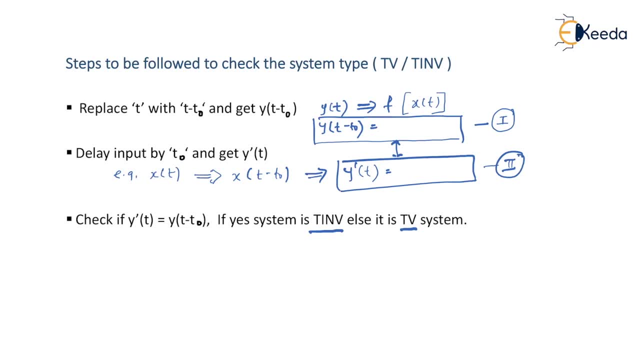 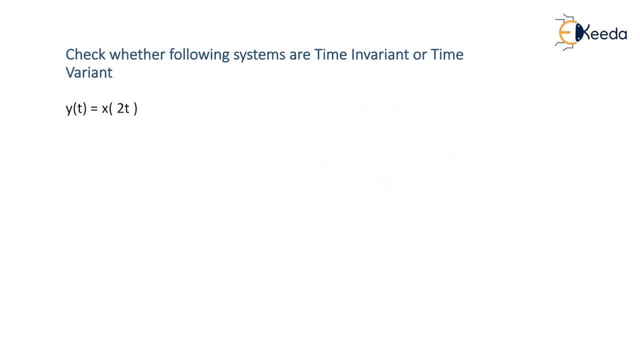 time invariant system. So if we start with the numericals then it would be quite clear to you. Question says: check whether the following systems are time invariant or time variant. The first question says y of t is equal to x of 2t. So we will be following the steps. Step number one says: 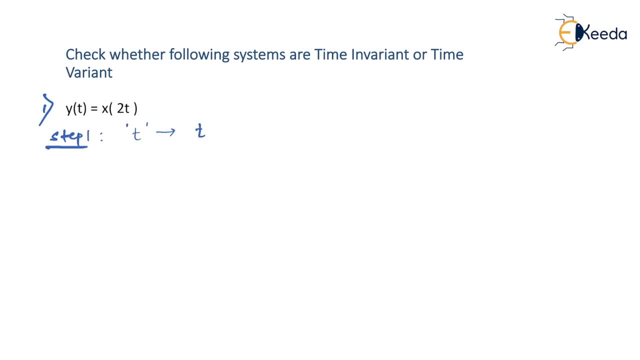 replace t with t minus t naught. So wherever you see t, just replace t with t minus t naught. therefore, on left hand side it will become y of t minus t naught and now it is equal to x of 2.. The bracket I will have t minus t naught. So if you open the bracket, y of t minus t naught is equal. 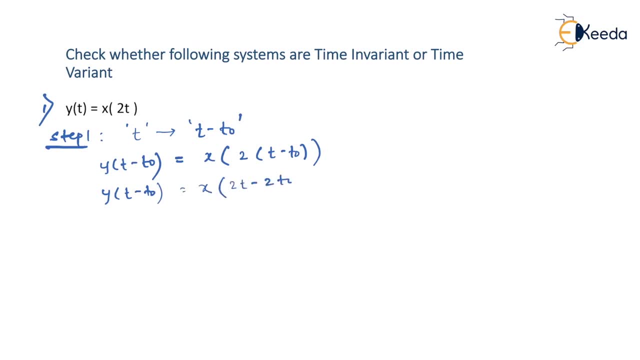 to x of 2t minus 2t naught. and now it is equation number one for us, right? Let us go for step number two. In step number two, remember you have to only delay input by t naught. Therefore, output becomes now y dash of t. 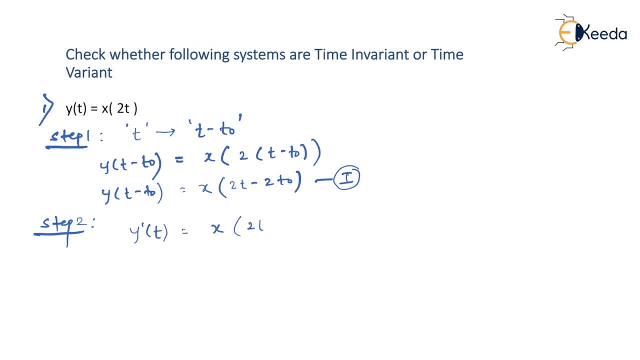 It is equal to x of. in the argument what is written? see carefully, it is 2t. then you have to delay it by t naught. So it is 2t minus t naught. So now it becomes equation number two. Remember, whatever argument is written over here, just subtract minus t naught from the given argument. 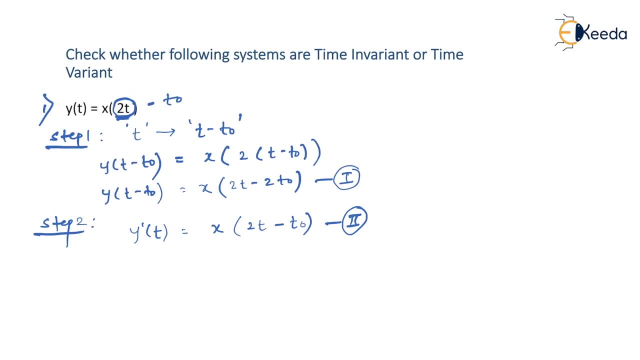 and that becomes y dash of t. and now, if you observe equation number one and equation number two, you can see clearly that y dash of t is not equal to y of t minus t naught. we know that if equal condition is present, it is time. 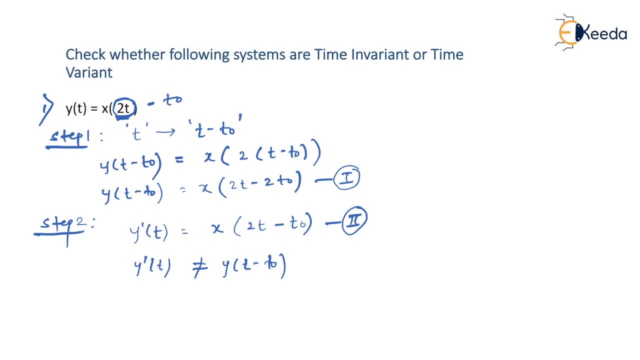 invariant system, else it is time variant system. so now the given system is time variant system. therefore it is time variant system. so in future, if you don't have to follow these many steps, then you can remember some shortcuts. see to it. what is done with the argument of x of t? original signal is x of t, but what is written? y. 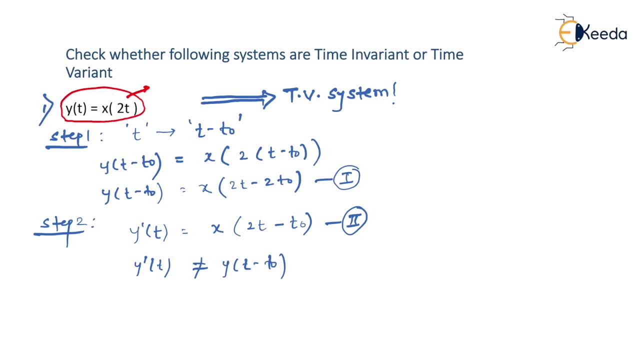 of t in terms of x of t as x of 2t. so what is done exactly? it is nothing but time scaling. remember: time scaling on the argument of x of t makes system time time variant. so you can just see whenever a time scaling is taking place on the argument of x of t. 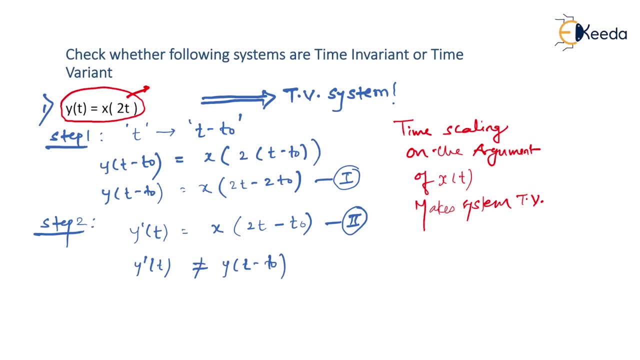 you just make sure that system is always time variant system right. so in future, if you just observe this, you can write the direct answer. instead of following so many steps, let's start with the next one now. it is: y of t is equal to x of minus t. let us see by following the number. 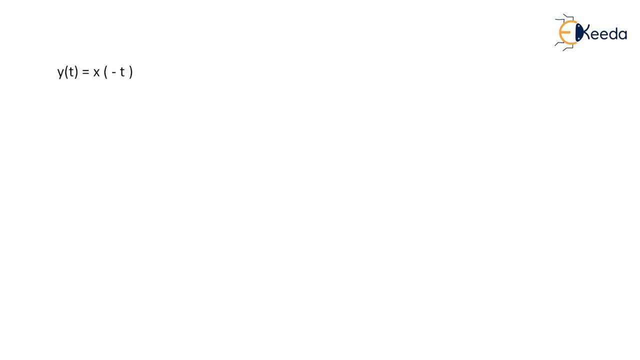 of steps to check whether the given system is time variant or time invariant. step number one is to replace t with t minus t naught. so it gives you y of t minus t naught. that is equal to x of now. we have a negative sign, so t has to be replaced with t minus t naught. 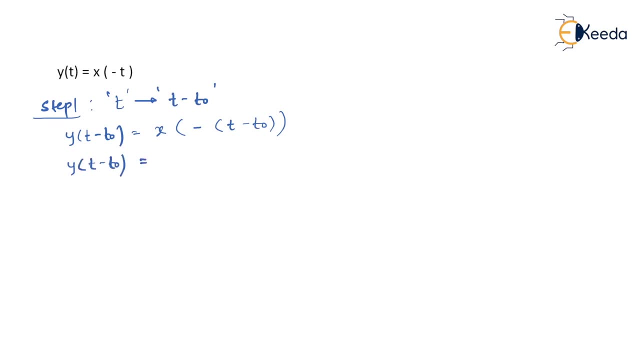 let us simplify this: y of t minus t naught. finally, i can write x of minus t plus t naught. right now it becomes equation number one for us. in step number two, you know that you have to delay input by t naught and you know very well whatever present in the 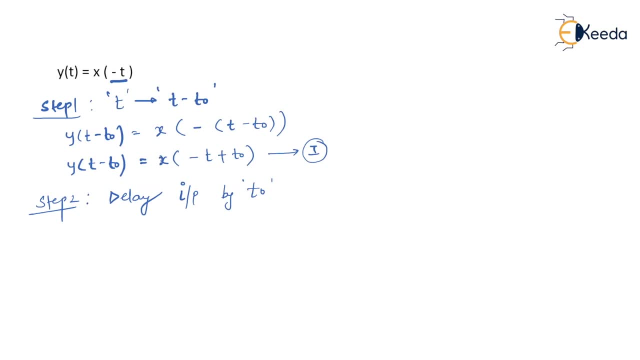 argument of x of t. just subtract t naught from it. therefore it gives you y dash of t, which is equal to x of minus t minus t naught. and now it is equation number two. observe carefully: equation number one and equation number two are again not same. 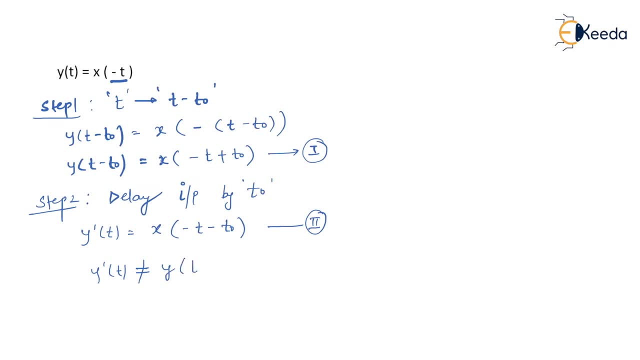 y dash of t is again not equal to y of t minus t naught, and it says that the given system is a time variant system. y of t is equal to x of minus t, where x of minus t is what we called as a time reversal property. all right, in fact, a time reversal property is a special case of time scaling only. 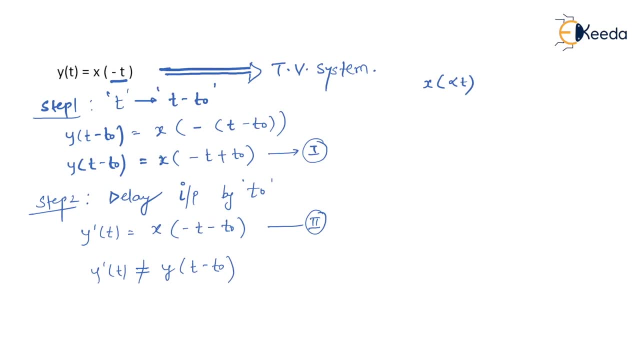 because for time scaling, what we write is x of alpha t of x of alpha t. if i now substitute alpha equal to minus one, it ultimately becomes x of minus t. right, and as we have already studied, whenever a scaling takes place on the argument of x of t, 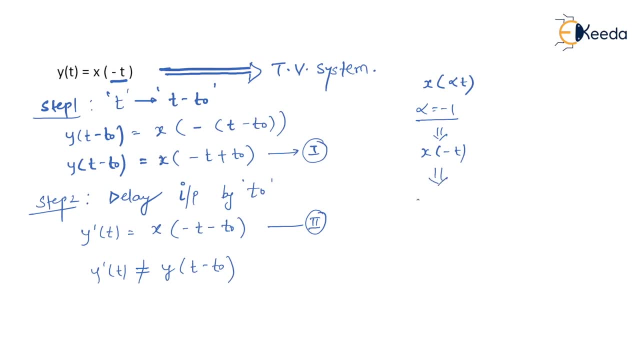 it always gives you a time variant system. therefore, it is a time variant system with respect to input variable x of t. if scaling is done, it always gives you a time variant system. now y of t is equal to x of t minus two. right, let us follow the steps. step number one replace: 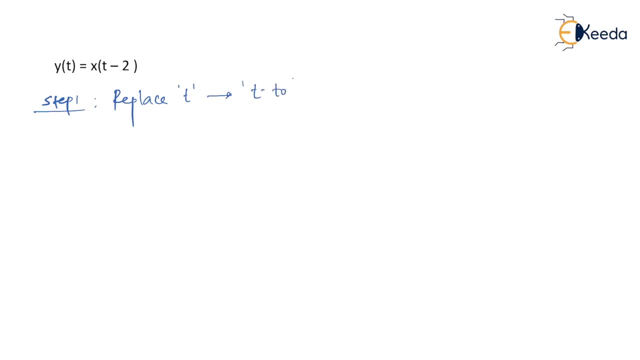 t with t minus t naught. so it gives you y of t minus t naught, which is equal to x of t minus t naught minus two. so it becomes equation number one in step two. and step two we just delay. we use y of t here to run over to x of t, right? so it gives us such that y of t is equal to y of t. 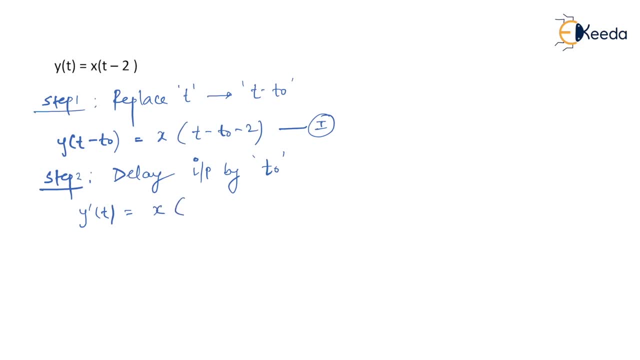 minus t. so what we are doing now we are CATCHing selfer the erf with cheers and we don't give you. so so are we. forth is equal to x of t with x of t with minus. that is ago and negative. so what we do is we keep the argument same. we just subtract minus t naught from it. i can rearrange like this: x of t minus t naught, i can write together and thereafter i can write minus two. also, the reason i am writing like this, so as to match up x of t minus t naught with minus x of t minus t, assure 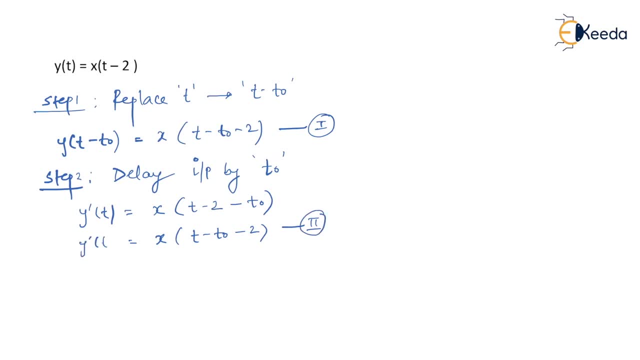 the reason why I'm writing like this: so as to match with equation number one. you can see clearly now: equation number one and equation number two are exactly same. so I can conclude: y dash of t is equal to y of t minus t naught, and whenever y dash 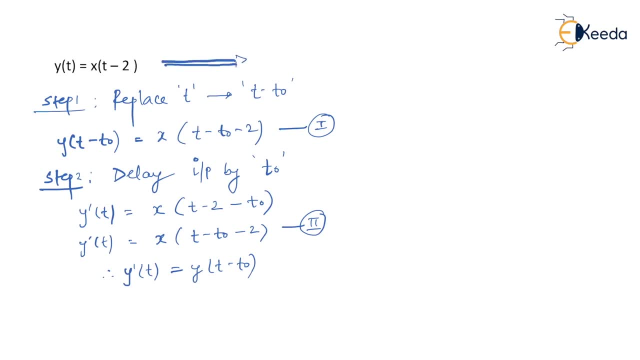 of t is equal to y of t minus t naught. so it is a time invariant system. now, if you observe what is done with variable t with respect to x, it is nothing but time shifting. so now you can conclude that time shifting. when you say time shifting, it can. 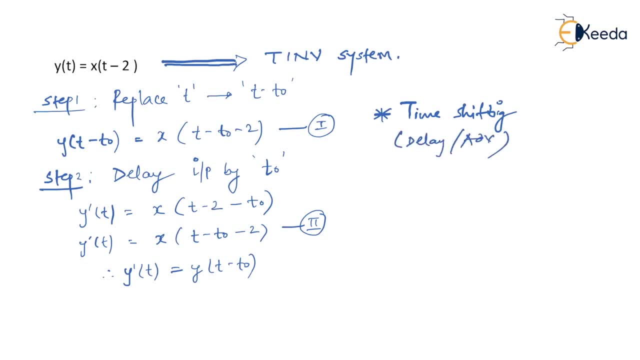 be delay or it can be advanced. also, it keeps your system as time invariant system. let us summarize what we have studied for a particular system. when y of t is expressed in, that is, x of t in any form with respect to x of t variable, that is t variable if time scaling is. 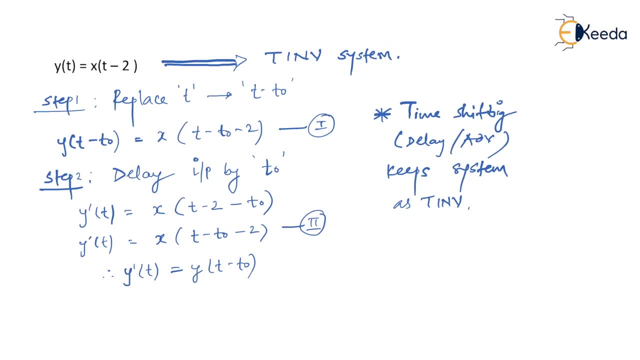 done or time reversal is done, then definitely it is time variant system. but in case, if time shifting is present, whether it is delay or advance, then it remains as time invariant system. so now, if you look at this sum, if only by observation, if i want to know whether the system is time, 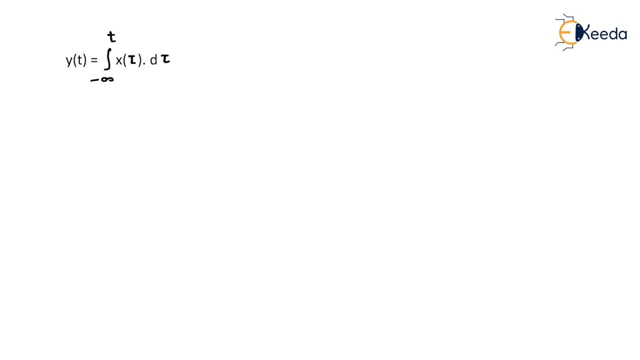 variant or invariant then? so this is actually an integrator system, right? so it is a system where x of t is input and y of t is output. so y of t is given as integration from minus infinity to t. x of tau, d, tau, right? so this is a perfect integrator system. so in this integrator system, 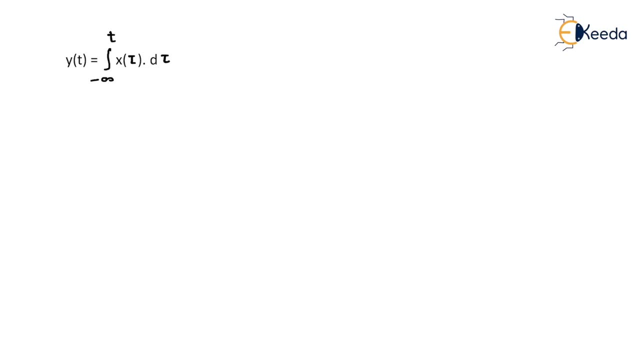 you have to see variable t, which is related to input. if you see t, neither time shifting is done or time scaling is done. therefore it is hundred percent time invariant system. but let us prove it by following a standard procedure. so in advance i know that it is time invariant system for sure. step number one: replace t with t minus t naught, so it becomes y. 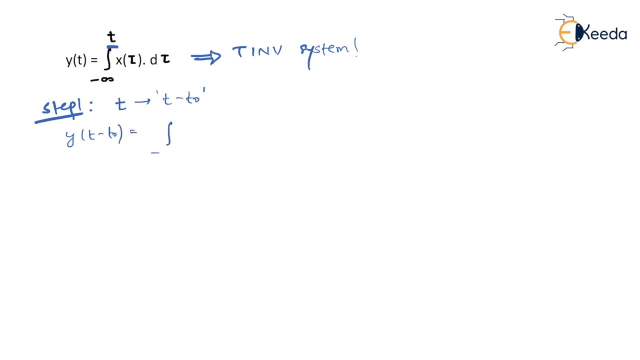 of t minus t naught, which is equal to minus infinity, to t minus t naught, x of tau, d, tau becomes equation number one. step number two: delay input by t naught, so it gives you y dash of t. lower limit and upper limit are not going to change because you don't have to really replace. 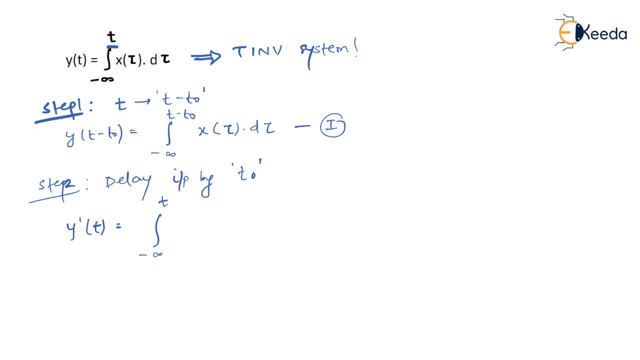 t with t minus t naught. you have to only delay input by t naught. so you know that what we used to do will be following the same. you have to only check what is argument of x and just subtract minus t naught from the given argument. 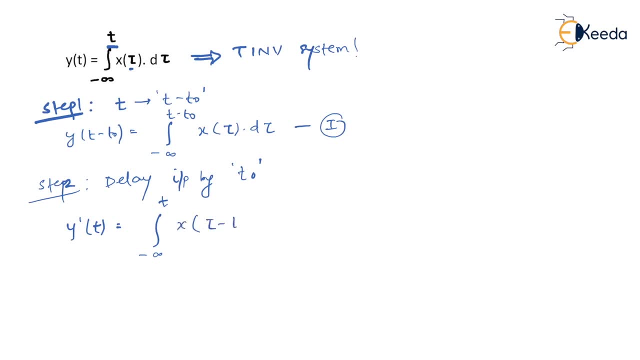 you have to only check what is argument of x and just subtract minus t naught from the given argument content. so it becomes x of tau minus t naught d tau. is that right? and now it becomes equation number two. if you observe equation number one and two, it gives you a feel that definitely. 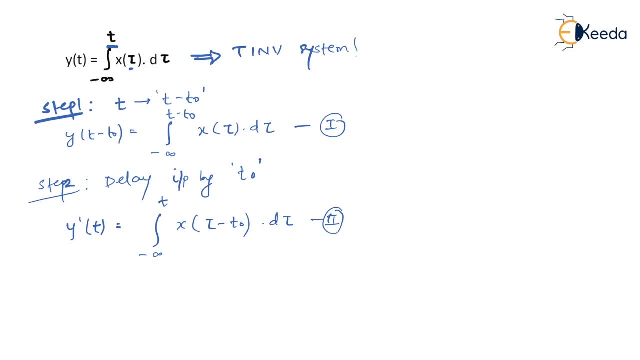 these two equations are not same and one might make a mistake to conclude as it is a time variant system. but let me tell you it is a time invariant system and i'll prove it. so how we are going to prove this. the reason why they are not seems to be equal: because 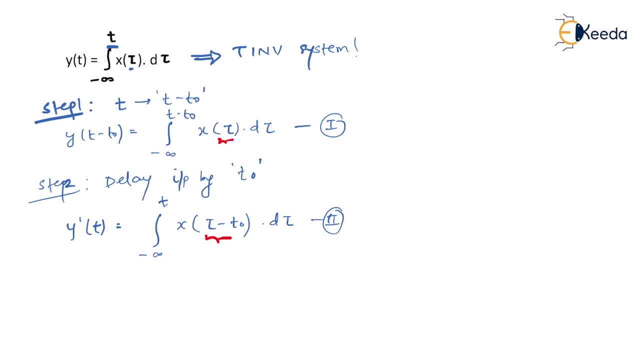 what we have in argument over here is tau, and what we have over here is tau minus t naught. let us assume we are replacing tau minus t naught with p, replacing tau minus t naught equal to p. so when i say tau minus t naught equal to p, then i can say that d. 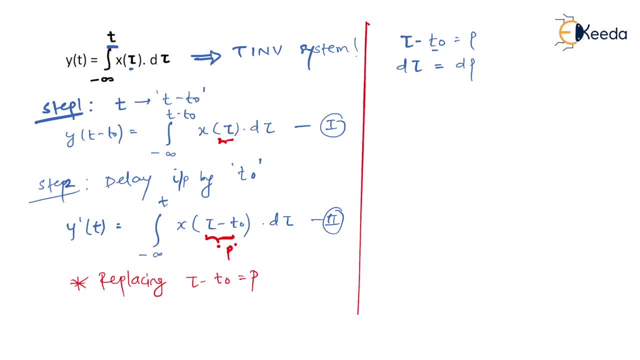 equal to dp because t? naught is constant. therefore derivative of t naught would be zero, only so d naught, so d tau equal to dp. now you know that you are going to replace this with p. okay, so d tau will become dp, right, but then you will have to check lower limit. 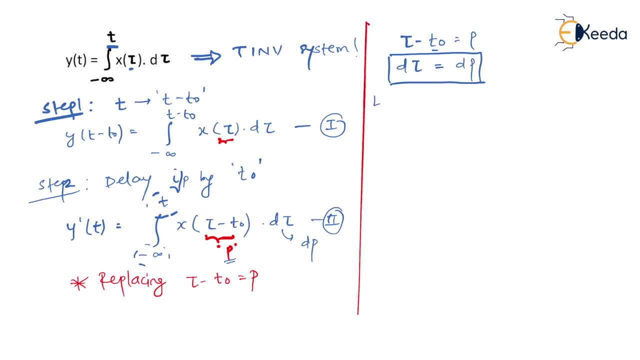 and upper limit also. so let us go for lower limit, calculation in lower limits we have. it was with respect to tau, so tau was equal to minus infinity. right, and what we have relation, as tau minus t naught equal to p. replace tau with minus infinity. so minus infinity minus t naught. 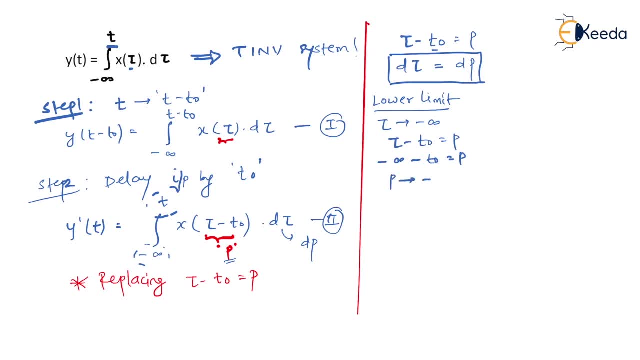 that is p. therefore p will remain minus infinity, only so lower limit remains minus infinity. let us take upper limit. so upper limit was simply t, so tau was equal to t, right, but now we have a near relation, that is tau minus. t. naught equal to p, replacing tau value equal to t here, so t minus. 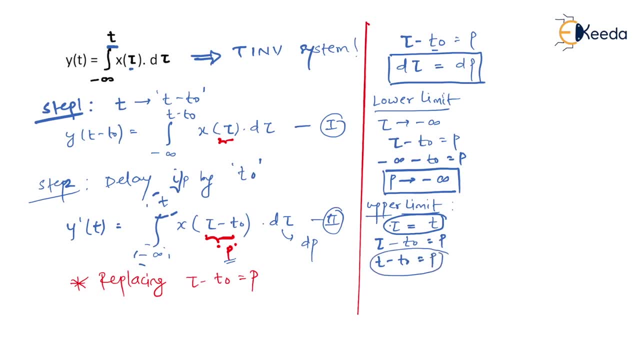 t naught becomes p. so new value of p is t minus t naught. so now this becomes lower limit and this becomes higher limit. okay, now we are going to change our equation of y dash of t, so y dash of t is equal to what is the lower limit? lower limit is minus infinity. 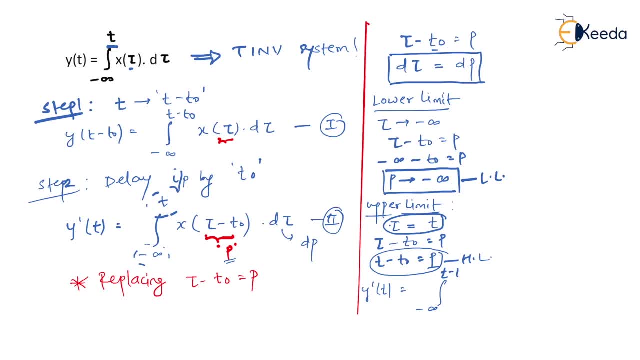 and what is the upper limit? upper limit is t minus t naught xo. what we had over here is tau minus t naught, which is replaced with p, and instead of d tau we have dp right now. if you see carefully, you have to make this as equation number three, and 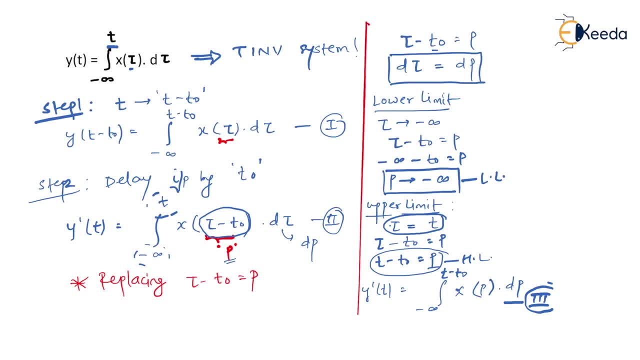 compare equation number 3 with 1. equation 3 and equation 1 are exactly same. now it may differ that what you find over here is tau and what you find over here is b. so let me tell you whether it is tau or whether it is p. it is just a dummy variable. so dummy variable can be anything right, but if you see, ultimately 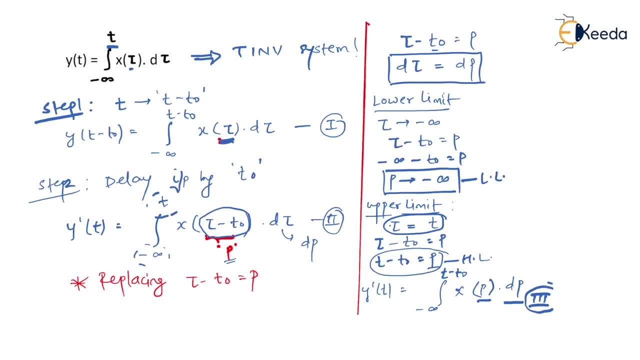 lower limit and higher limit are exactly same, with tau as a dummy variable in equation 1 and p as a dummy variable in equation 3. it really doesn't matter. therefore, i can say that equation number 1 and equation number 3 are exactly same. that is, y dash of t is equal to y of t minus t naught. 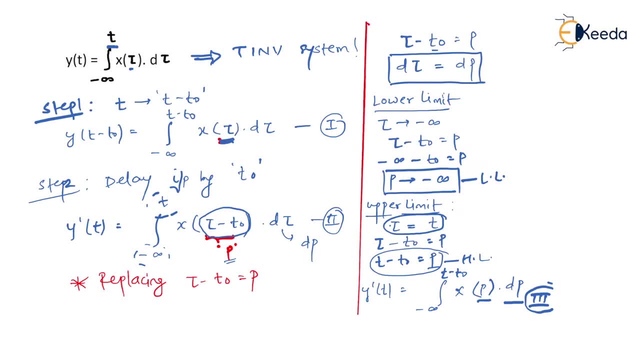 therefore the given system is time invariant system. but if you really don't have to go through a huge procedure, then you have to really remember certain tricks, and those tricks are: you have to always check variable t with respect to input, right? so here neither scaling is done nor shifting. 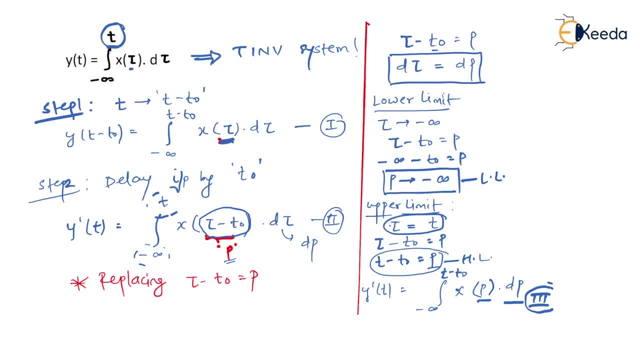 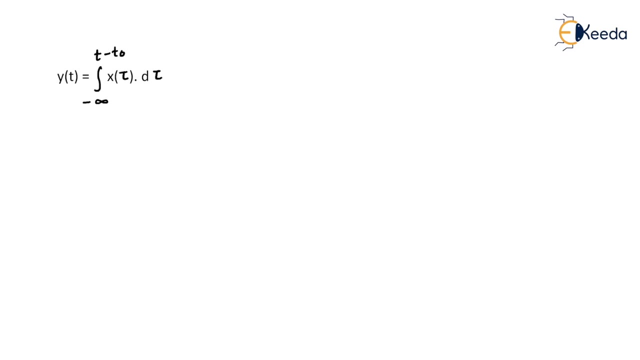 is done. and let me tell you, shifting really doesn't matter, because only if shifting is done it remains time. invariant system only. this is what we have already seen with an example, right? so let's see the next example. example says: y of t is equal to integration from lower limit as minus infinity upper limit is.